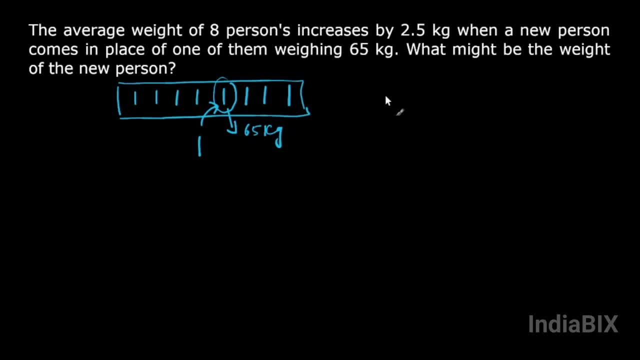 weight of the group increases by 2.5 kg. Let us suppose the initial average weight of the group was Average weight. initial was x. Now, after this change, average weight of the group becomes Average weight final: It increases by 2.5 kg. 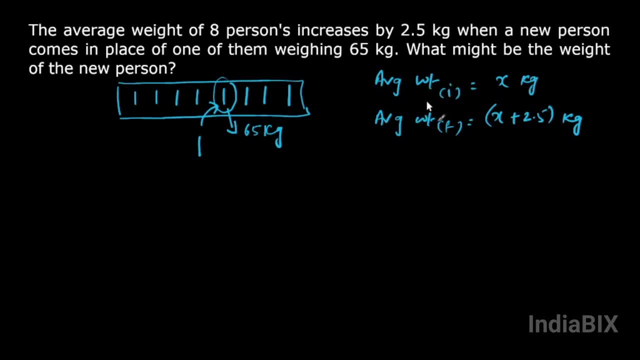 Ok, Ok. So we have to find, according to the given condition, the weight of the new person. We know the formula of average Average is sum of all the entities by number of entities. Here the number of entities are 8, because there are 8 members Before and after the. 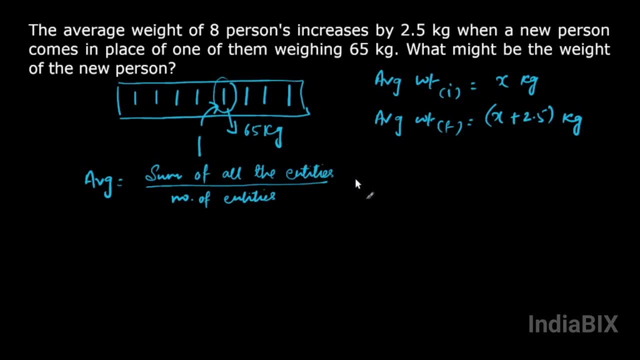 replacement. Let us suppose the sum of all the entities before replacement be Y And we have assumed the average of the group, average weight of the group before replacement, is x And the So x will be equal to y by 8 and therefore y will be equal to 8x. 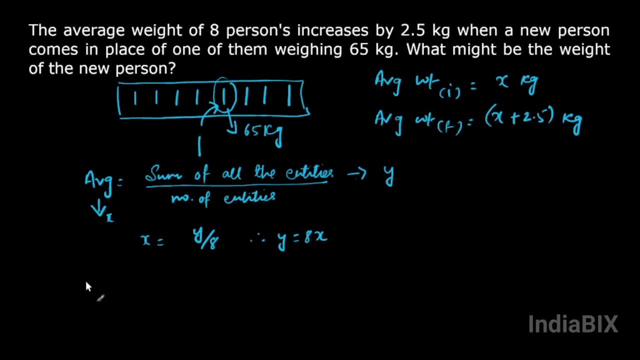 Now let us see what is happening after the change. After the replacement, average weight of the group increases by 2.5 kg and sum of all the entities y, and the person whose weight is 65 kg gets replaced and a new person comes in the group whose weight we don't know. 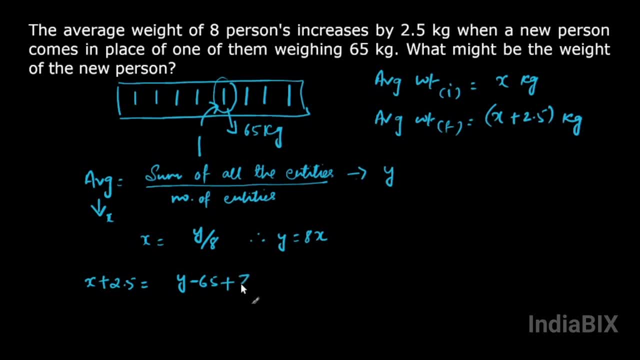 Let us suppose the weight of that person, the new person, be z, and now also the total number of members remain 8, because one goes and one comes. Now doing the cross multiplication, 8x plus 2.5 into 8 is 20..